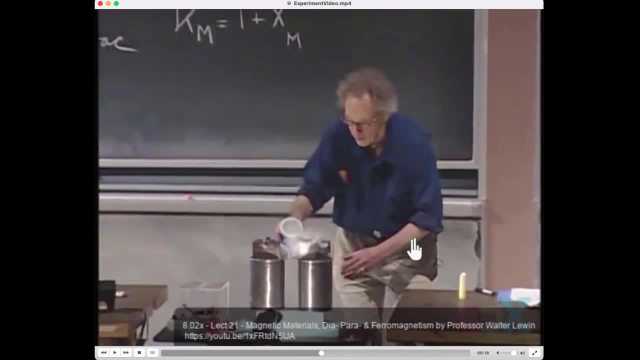 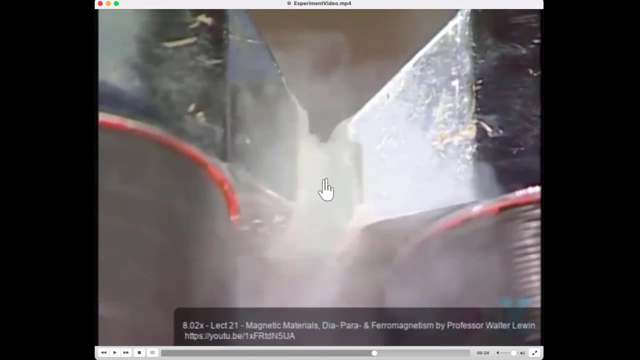 Okay, let me show you another, another one. This is a demo by the famous Professor Walter Lewin at MIT. He's pouring liquid oxygen into an electromagnet. See what happens There. we go, Look at what you see. You see that liquid oxygen sticks, sticks to the magnet, meaning it gets attracted to magnet. What's going on? Why are these things attracted and repelled to magnet? They shouldn't be, isn't it? 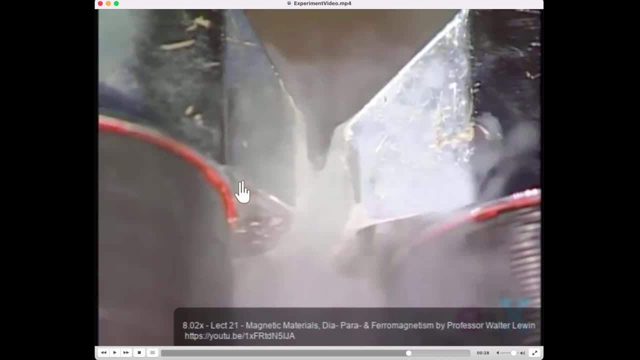 Well, it turns out that most materials are actually either slightly attracted or repelled by magnets. So with careful experiments you can actually see that. But what's mind boggling to me is whether it's attracted or repelled depends on and get this. 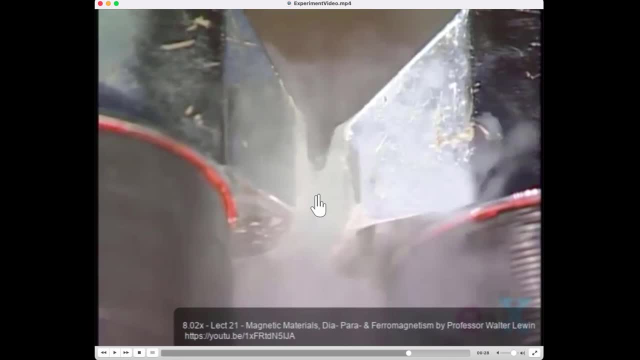 it depends on whether the atoms of that element have paired electrons or unpaired electrons. But why? How does that decide whether something is attracted or repelled by a magnet? Well, let's find out. We've already seen that atoms tend to have magnetic moments because of electrons. 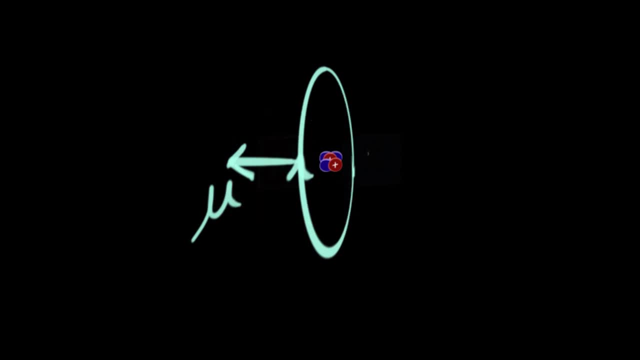 going around forming current loops. Current loops give magnetic moments, which basically means they act like tiny tiny magnets. But most atoms have more than one electron And the electrons tend to pair up. Now, whenever electrons pair up, you can imagine that the two form current loops in the 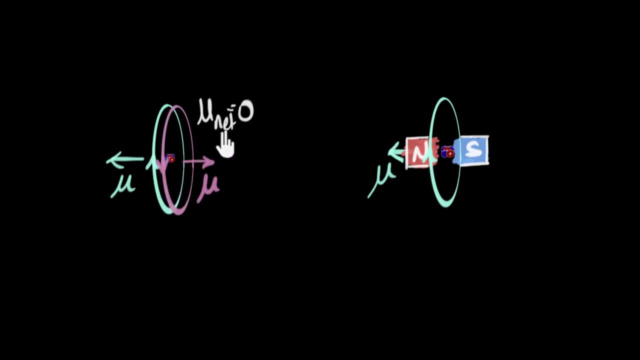 opposite direction, giving the net current zero. so their magnetic moments cancel out. So this means if you have atoms where all electrons are paired up and their magnetic moments cancel out, they do not behave. these atoms do not behave like a magnet. So this means that if you have atoms where all electrons are paired up, they do not behave. these atoms do not behave like a magnet. 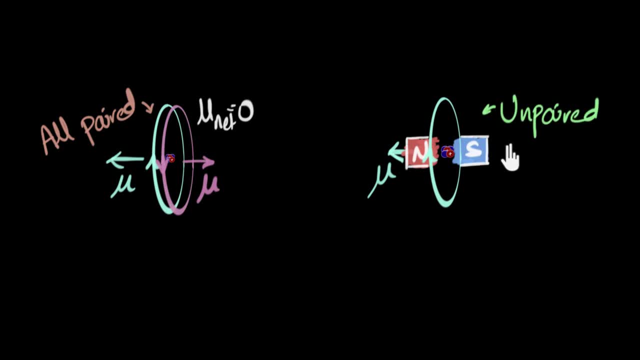 like tiny magnets. On the other hand, if you have, at least if the atoms have, at least one unpaired electron, then they will generate some magnetic moment and these atoms do behave like tiny magnets. Now let's see what happens when you bring a magnet close to them. 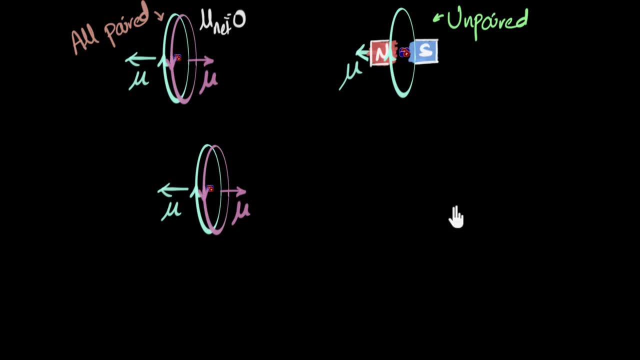 So let's start with the atoms that are completely paired up. What would happen if I were to bring a giant bar magnet close to it? My first thoughts are: these atoms do not behave like tiny magnets, right, And so they should be completely unaffected. 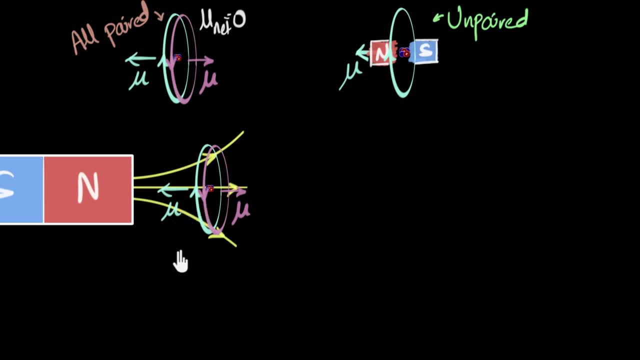 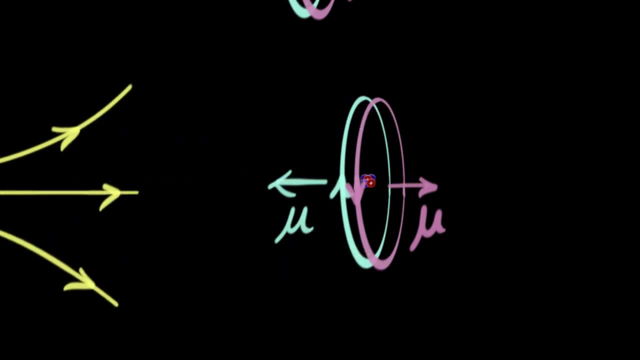 by magnetic fields, So nothing should happen, right? Well, don't forget about electromagnetic induction. And you might be like: what, what are you talking about? When I brought the magnet close to this, the magnetic flux through these loop changed. 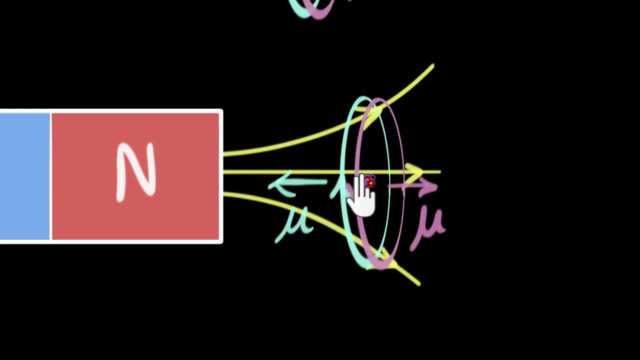 And we know from Faraday's law that now there will be an EMF induced in these current loops which tends to oppose that change, Lenz's law, And so there will be an EMF induced that tends to oppose the field, which means the EMF will be induced in this direction. 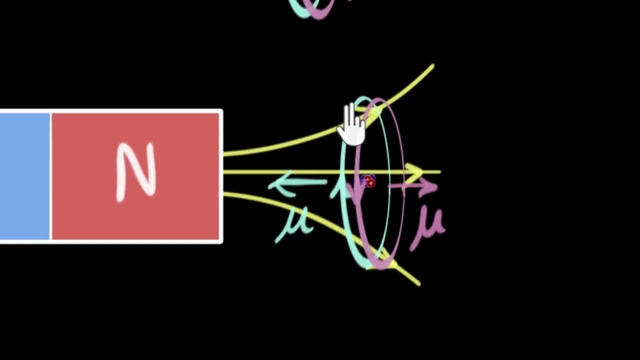 the blue current's direction. So what that means is that induced EMF strengthens this current. So I'm gonna show this current a little bigger, that this current becomes stronger because of the induced EMF, But this current becomes a little weaker because the induced EMF is in the opposite direction. 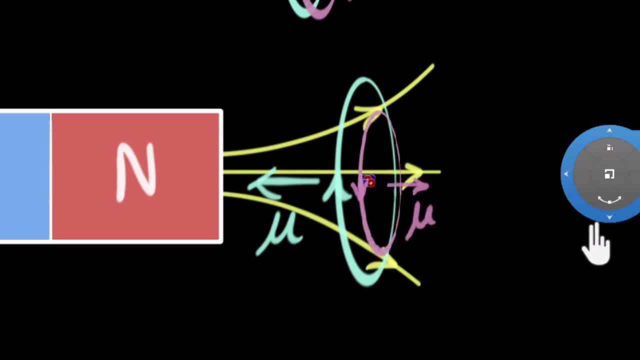 to this current, And so the current now becomes a little weaker And, as a result, look, they're no longer going to cancel each other out. There's gonna be a slight difference. The dysmagnetic moment is slightly different. It's slightly higher than this one. 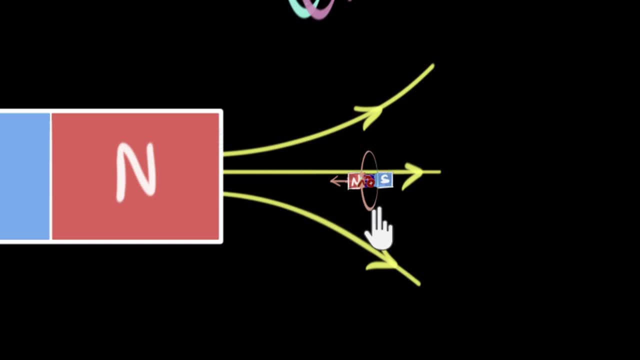 And so there is a small magnetic moment induced and starts behaving like a tiny magnet. And so look, due to Lenz's law, the atom starts to behave like a tiny magnet, And look at how it's oriented in the opposite direction. 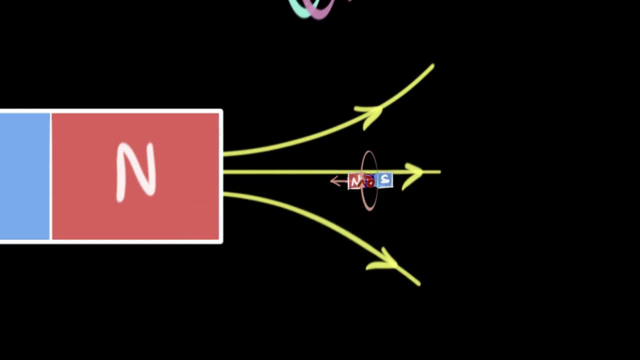 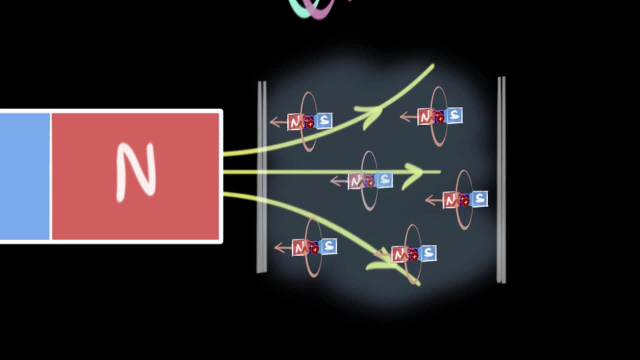 So is it gonna attract or repel? It's gonna start repelling it. Same thing is happening in the water. Water molecules are all paired up, but when you bring a magnet close to it, due to induction, they behave like tiny magnets. 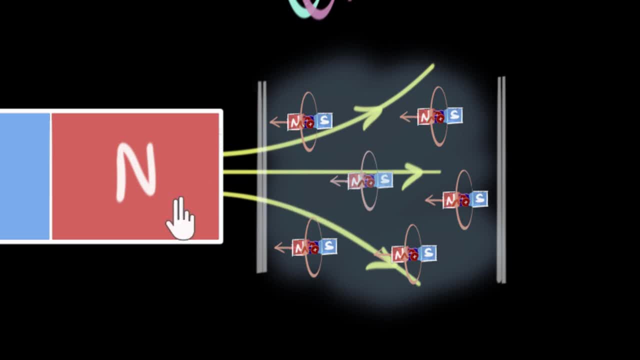 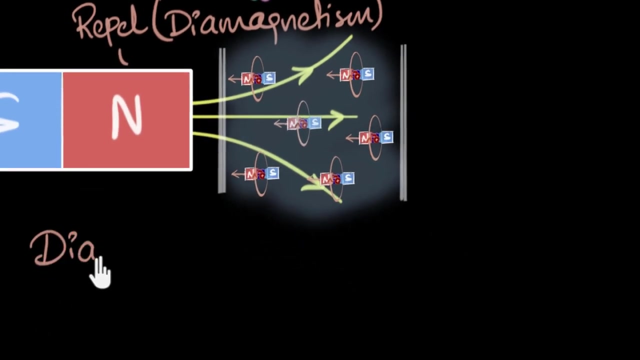 And, as a result, the water gets slightly magnetized in the opposite direction and ends up repelling the magnet. This phenomena, where atoms starts repelling the magnetic field due to induction, is what we call diamagnetism, And such materials like water are called diamagnets. 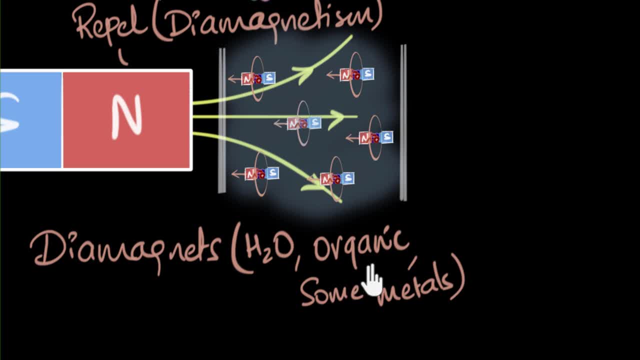 And the examples include water, of course, and a lot of organic substances like you, me, wood. all of us are diamagnetic. Living beings are all diamagnetic, And there are some metals as well, which we'll get back to towards the end of the video. 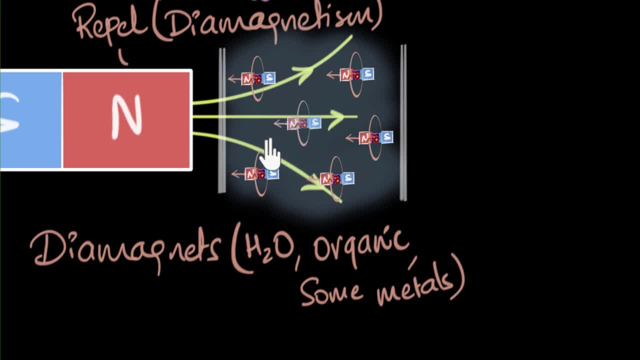 And although diamagnetism is a very, very weak property, which is why you should do very careful experiments to see that if the external field is strong enough, the force, the repulsion could be strong enough and you can use that to levitate things. 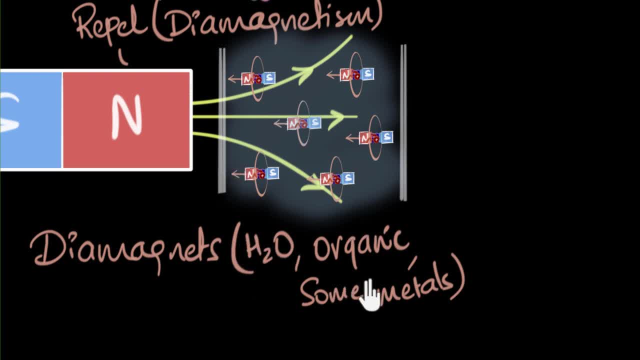 And so, for example, if you bring this bar magnet from a giant magnet from the bottom and put a frog on top of it, it has been done. The frogs tend to levitate because of the diamagnetism. The repulsion can be stronger than gravity. 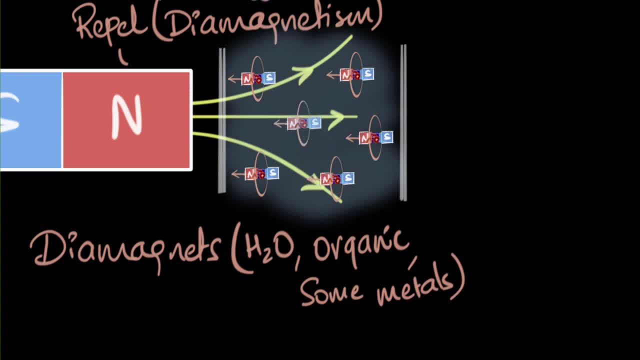 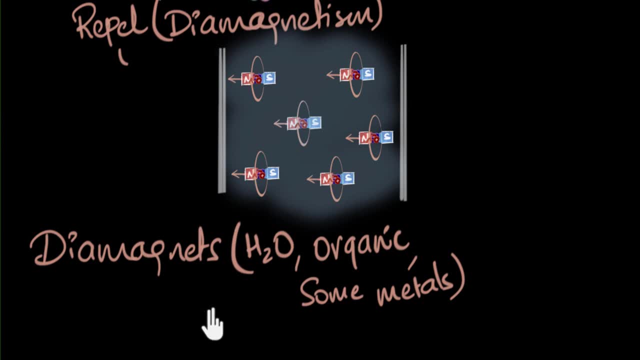 You can check out some videos of frog levitating by magnets. Pretty cool. But now here's my question for you: What would happen if I were to take that magnet away? Do you think that this magnetized water would stay magnetized now? 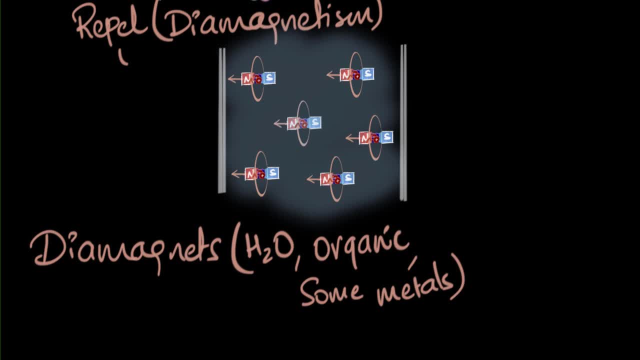 or something else. something would happen to them. Can you pause and think about it? Okay, again, electromagnetic induction will take place, but this time because the magnetic flux is decreasing. you'll try to increase it from Lenz's law. 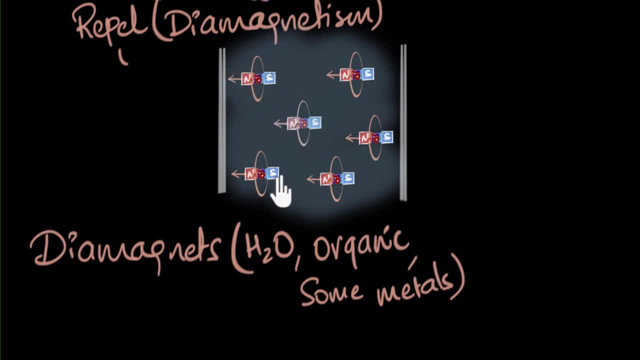 so there'll be induction happening in the opposite direction. This will completely kill this current and the water would lose its magnetism. So diamagnetism is not only weak, but it's also a very temporary phenomena. Okay, now let's consider materials. 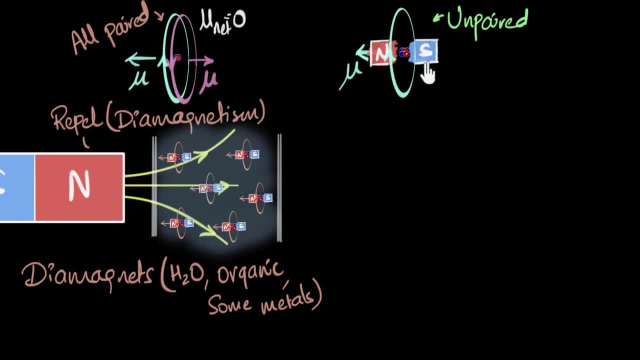 whose atoms have these permanent dipoles, They do behave like tiny magnets. Oxygen is an example. So an immediate question to me is: why does an oxygen behave like a magnet? Because the atoms of oxygen do behave like magnet right. Well, if you could look at the magnet right. 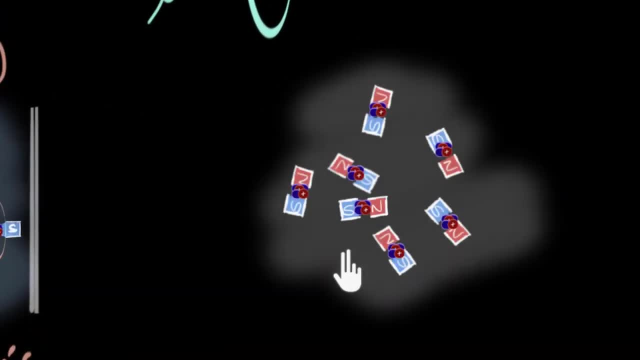 If you could look at all the atoms inside, say, oxygen, what you'll find is that their magnets. these magnets are all randomly oriented, And so, although each atoms do behave like tiny magnet as a whole, all their magnetism gets completely killed. 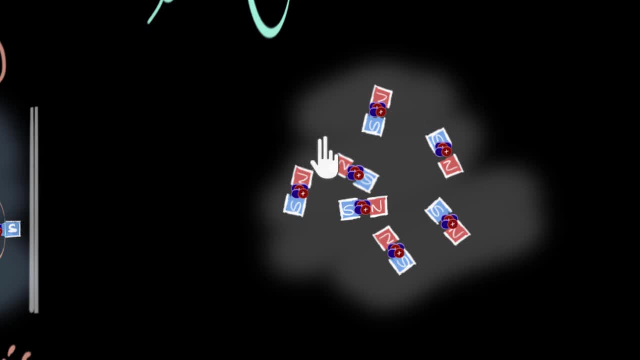 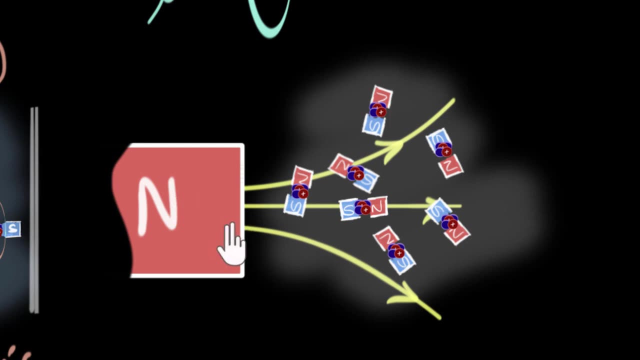 because of the random orientation, and so oxygen as a whole still doesn't behave like a magnet. But now what do you think will happen if we bring it close to a magnetic field? Well, the magnet starts putting a force on these tiny magnets. 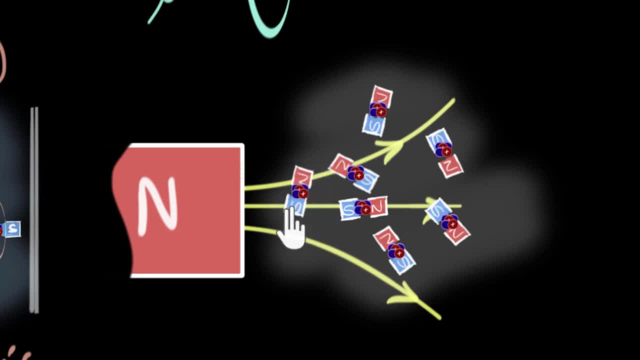 If you look over here, the north pole gets repelled, the south pole gets attracted and, as a result, it'll turn. So all these tiny magnets tend to turn and get aligned in the direction of the magnetic field, And because of this it's no longer random. 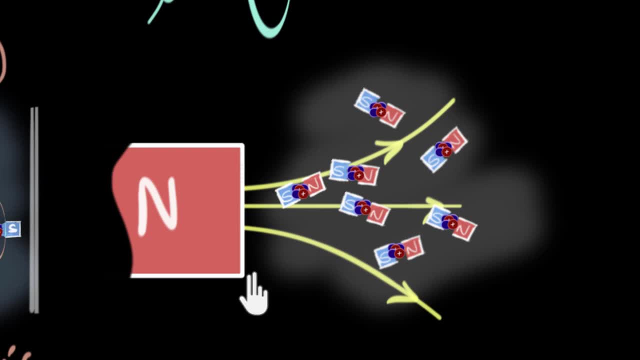 Pretty much. this side is now behaving like a north, this side is behaving like south, and now the oxygen has been slightly magnetized. This material is slightly magnetized, But look in what direction it's magnetized. This is south, means it's attracted. 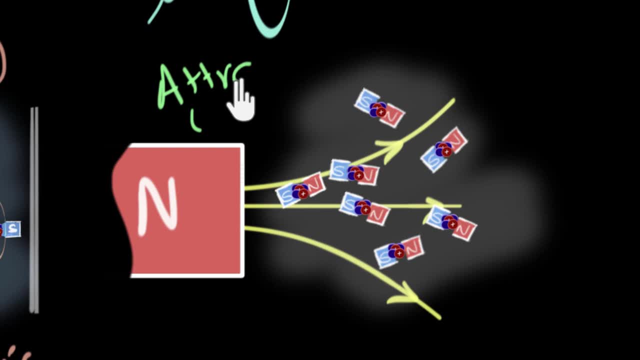 And this phenomena, where materials attract magnets, is what we call paramagnetism. Paramagnetism- You might say that they're not completely aligned, mainly because there is a lot of thermal agitation. These things are all vibrating, So they're somewhat aligned, which means that paramagnetism is also very, very weak. 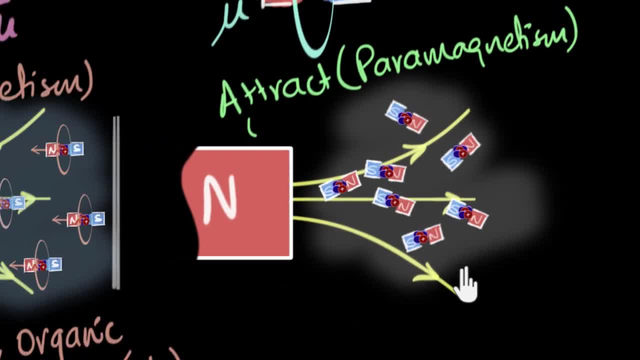 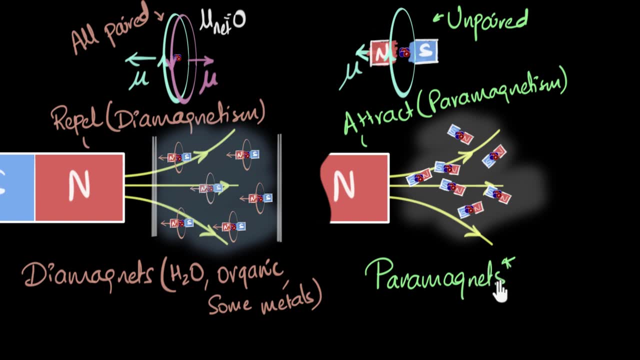 and again. we need careful experiments for this, And such materials that get weak, equally attracted by magnets, are called paramagnets, And I'll put a star over here- mainly because not all materials that have unpaired electrons behave like paramagnets. 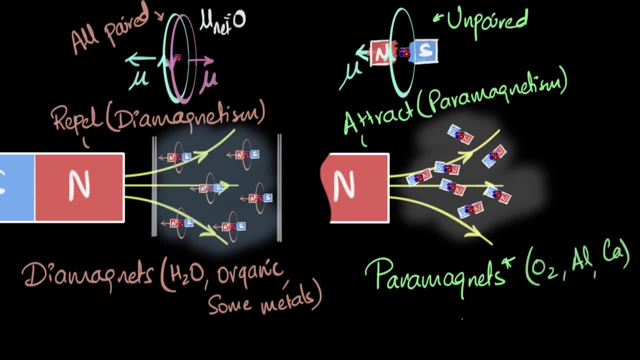 We'll get back to that towards the end of the video, But anyways, the examples include, of course, oxygen, and now you know why oxygen got stuck in that magnet: mainly because it's a paramagnet. But other examples include aluminum calcium. 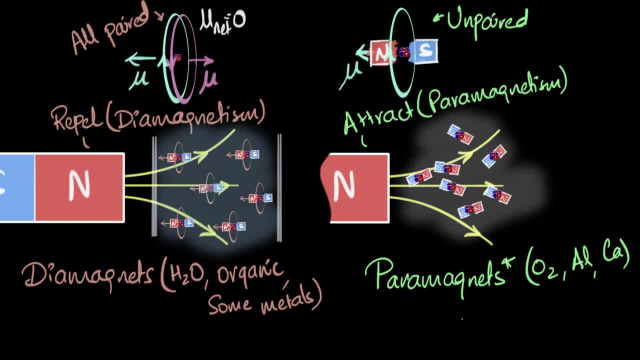 and I'm sure there are other examples out there. And again the same question over here: what would happen if I were to get rid of that magnet? Would oxygen stay magnetized? Well, now, there's no reason for them to stay magnetized. 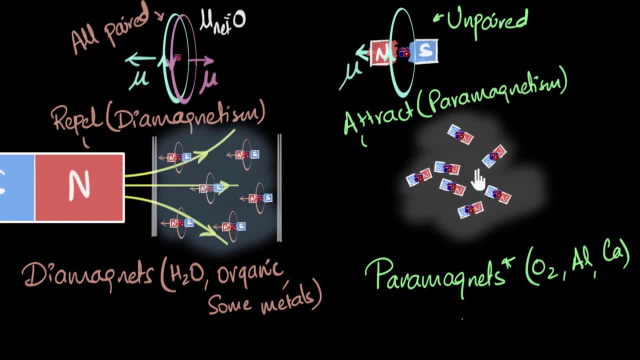 because, remember, all these atoms are jiggling and vibrating randomly, and so what will happen is they will go back to how they were before and it will lose its magnetism. So again, paramagnetism is a very weak and it's also a temporary phenomena. 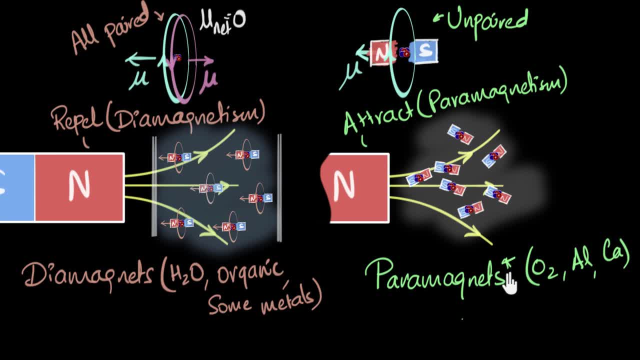 So now, before we move on to that last part where I put the asterisk over here, can you pause and differentiate between diamagnetism and paramagnetism? See what differences and similarities do you see? All right, So first of all, this repels and this attracts. 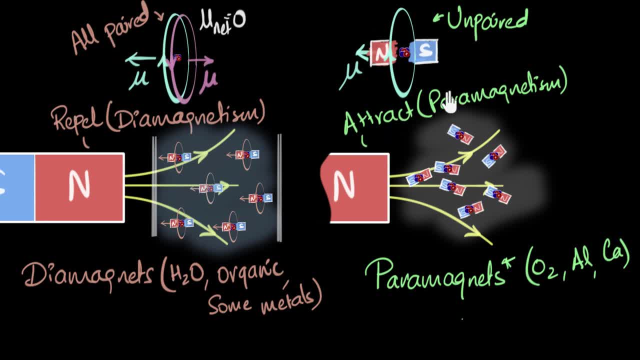 Secondly, this works on paired electrons. This is on unpaired electrons. Here we have temporary dipoles induced in the opposite direction. Once you get rid of the magnet, the dipoles are gone. Here you have permanent dipoles that are turning. 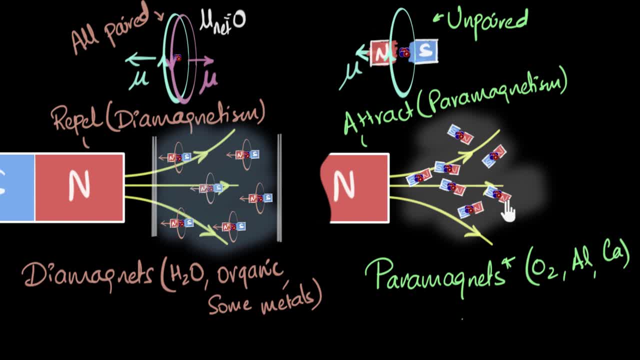 due to the magnetic field. Another important question is: how does temperature affect them? So let's look at paramagnetism first. What do you think would happen if I were to lower the temperature, reduce the temperature? Do you think the paramagnetism would get stronger, weaker? 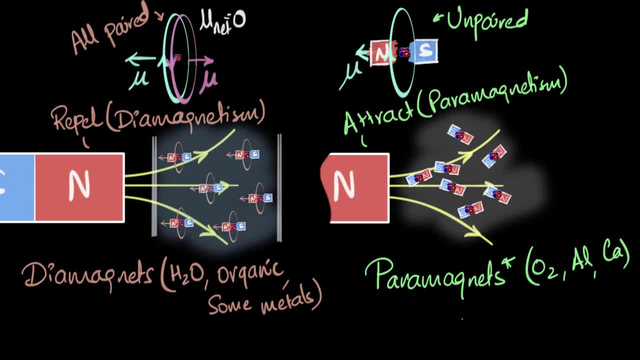 or do you think it wouldn't change? Can you pause and think about it? Okay, We saw that paramagnetism happens due to alignment. The more alignment, the more paramagnetism. right, But remember, the enemy of the alignment is the thermal vibrations. 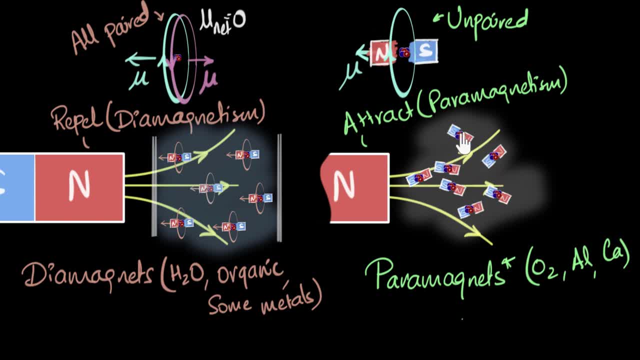 More thermal vibrations, harder it is to align. So, at higher temperatures, more thermal vibrations, harder it is to align, less paramagnetism. And that's why, when you lower the temperature, you get higher paramagnetism. In fact, that's the reason why liquid oxygen 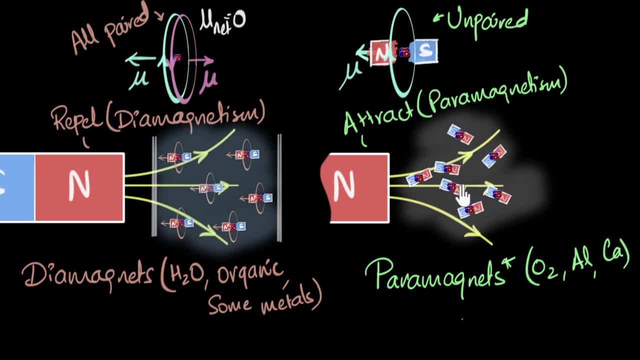 is highly paramagnetic compared to gas oxygen because it has a much lower temperature, And of course it's also because liquid oxygen has more density, more atoms per cubic meter, more attraction. But anyways, what about diamagnetism? How do you think it changes with temperature? 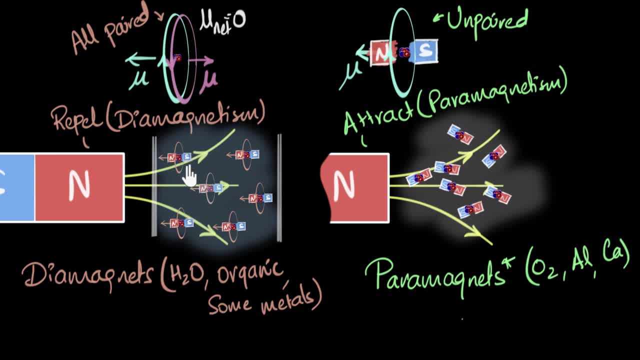 Well, diamagnetism does not depend upon the vibrations of the atom at all. It is due to the currents induced. right, The currents induced does not. does not depend on whether the atoms are vibrating or not vibrating, and therefore diamagnetism is pretty much independent of temperature. 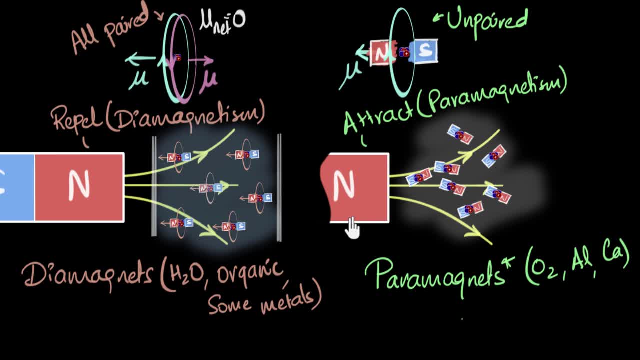 So that's another big difference that you see. What similarities do you see? Well, they're both pretty much weak and they're temporary phenomena, and that's where ferromagnetism is different. Ferromagnetism, you can retain the magnetism. 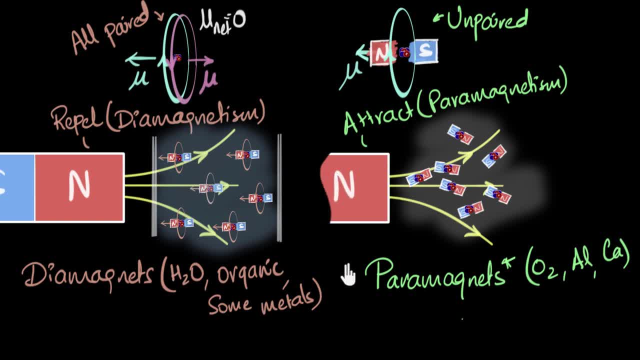 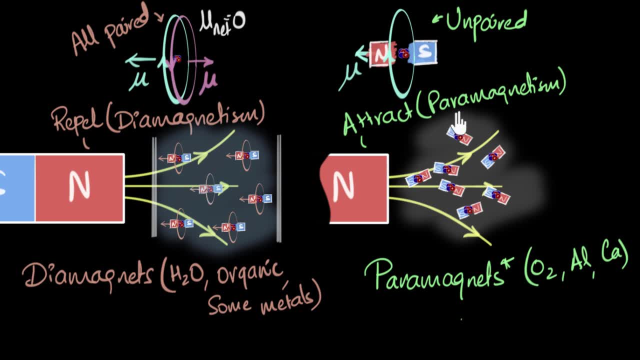 even after you remove the magnets, But they're so cool they deserve a video of their own. so let's not talk more about ferromagnets here. Finally, I said that not all materials whose atoms have unpaired electrons behave like paramagnets, and I'll give you examples. 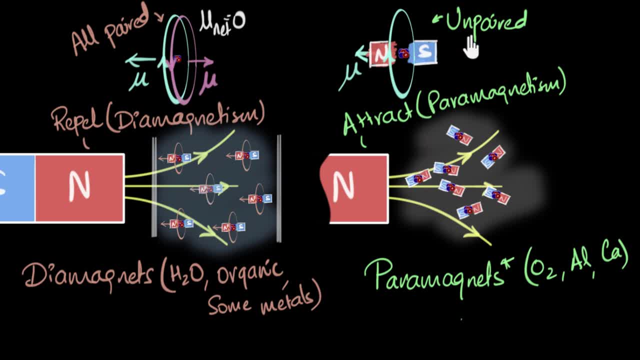 Copper, gold, silver- they all have an unpaired electron. They do not behave like paramagnets, They behave like diamagnets. Why do you think that happens? Can you pause and come up with a theory for that? Okay, here's a big question for you. 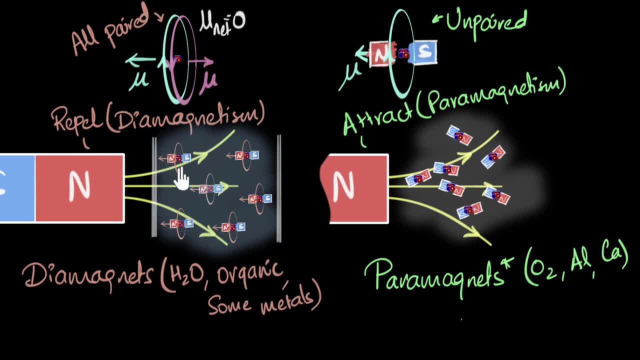 Whatever we saw over here, the whole electromagnetic induction causing diamagnetism- shouldn't that happen here as well? I mean, even this also contains paired electrons. inside All atoms have some or the other paired electrons, inner electrons, So shouldn't they undergo diamagnetism? 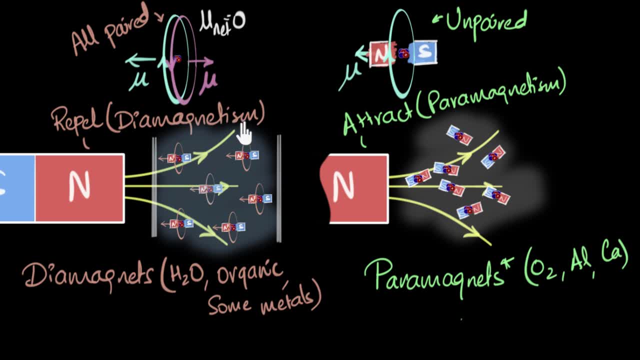 Same phenomena? right, They do. Diamagnetism is a universal phenomena. You can find that in every single material, whether it is iron or oxygen or aluminum, doesn't matter no differentiation. Every material have some or the other degrees of diamagnetism.